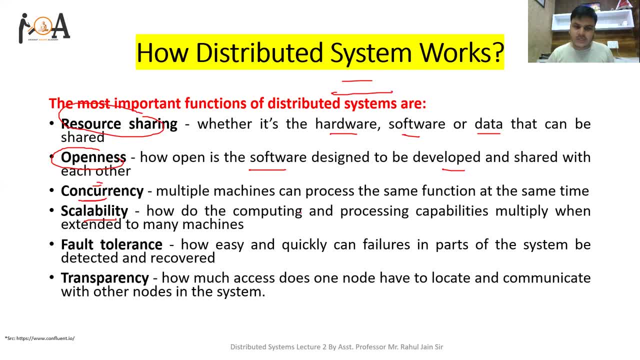 earlier as well. scalability: how do the computing and processing capabilities multiply when extended to many machines? fault tolerance: how easy and quickly can failures in parts of the system be detected and recovered? suppose we are sharing resources and suppose one resource link is failed or one component is failed or one node is get failed. then how quickly and how frequently we. 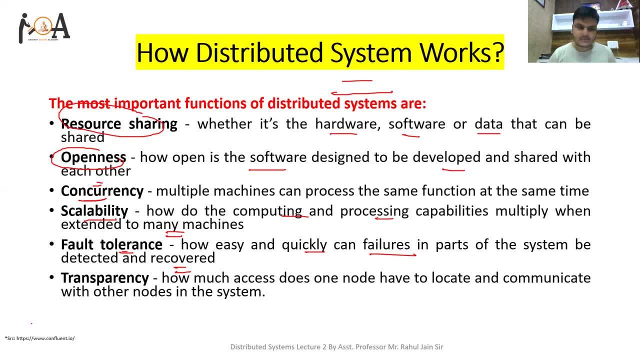 are recovering the failure parts right. that is the fault tolerance and the transparency that. how much access does one node have to locate and communicate with other nodes in the system? so this is how togetherly distributed systems works. on this point right now, the next one here is: 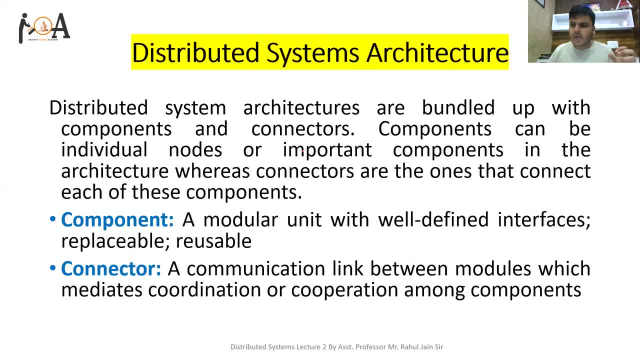 distributed system architecture. so if you talk about basics of distributed system architectures, distributed system architectures are bundled up with components and connectors. what points are here, components and connectors? components can be individual nodes or important components in the architecture, whereas connectors are the ones that connect each one of these components. so let's say we have a node 1, we have 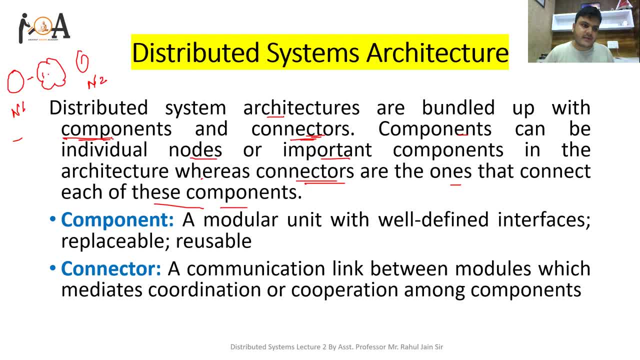 node 2, connected via a network. they are connected via a network. So this node one and node two, they are called as components, Okay, And these connectors, which is connecting that node to this components, to this particular network. this would be called as connector, Okay. So 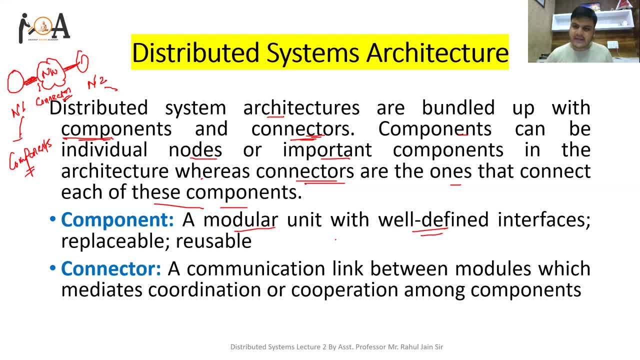 component. it is a modular unit with well defined interfaces which are replaceable and reusable, and connectors: a communication link between modules, a communication link between modules which may be at coordinate or corporation among components. So it will mediate the coordination and cooperation among components. So they are connectors. Okay, 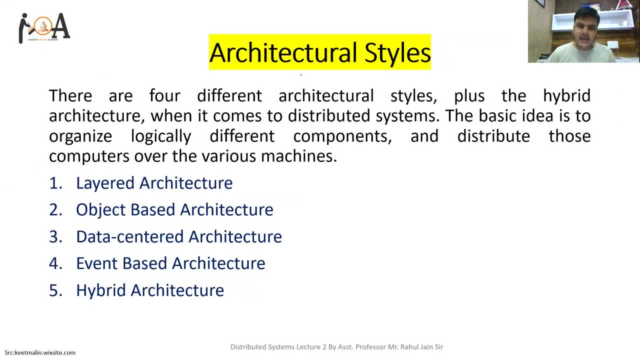 Now let's discuss about architectural styles. architectural styles: There are basically four different architectural styles, like a layered architecture, object based architecture, data centered architecture and event based architecture, But we also have a plus hybrid architecture when it comes to the distributed system. So, again, the basic idea is to organize logically different components and distribute. 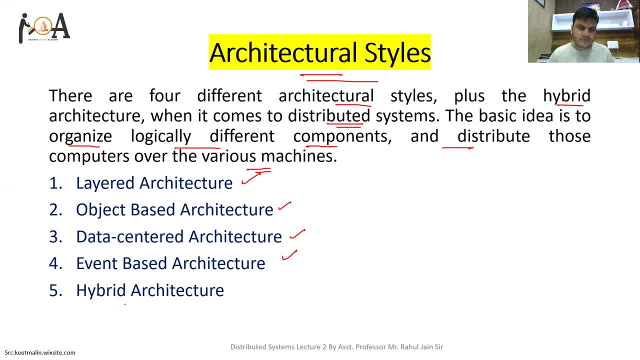 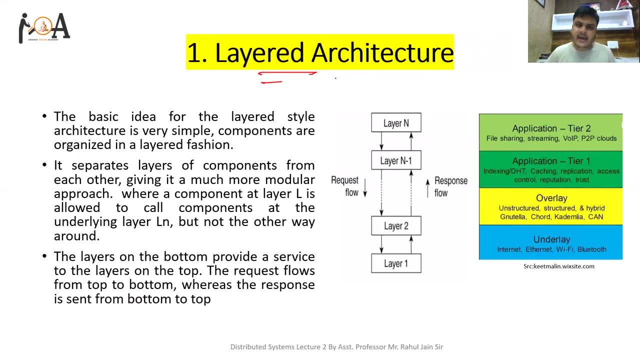 those computers over the various machines. So we have hybrid architecture also. So let's discuss the first type of architecture, that is, the layered architecture. So if you will see the first point, the basic idea for the layered style architecture is very simple. The components are organized in layer division. you can see here the components. 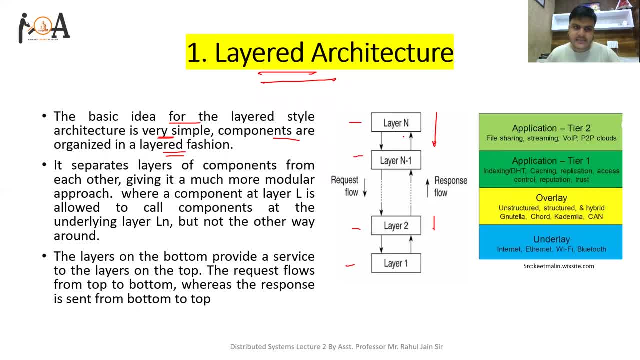 are fashioned here in layer division, the components here organized layer division, similar to OSI model, similar to OSI model in computer networks, layer by layer, layer by layer. style is there and each layer can communicate to its upper layer and down layer, like that right so layer it separates layer of components from each other, giving it much. 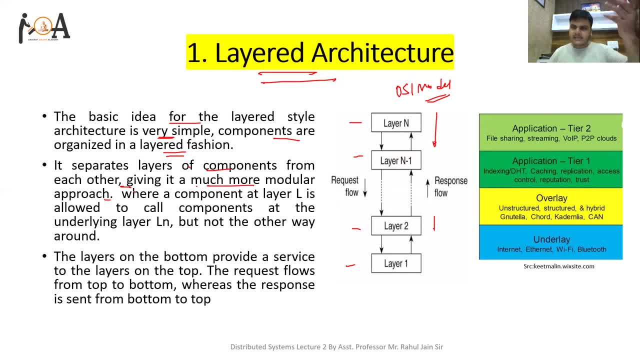 more modular approach. modular approach means they can communicate via, like this, request flow and response flow, like that where a component layer l is allowed to call components at the underlying layer l but not the other way around. let's say, in a osi model we have physical 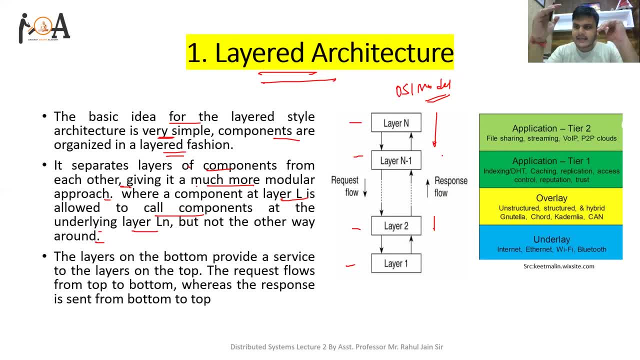 layer which can communicate to the upper layer right, data link layer. and data link layer further can communicate to network layer and network layer can communicate to transport layer and network layer can also communicate to data layer. but network layer directly can't connect to physical layer right. so in the, in same manner, in same manner, this layer architectures. 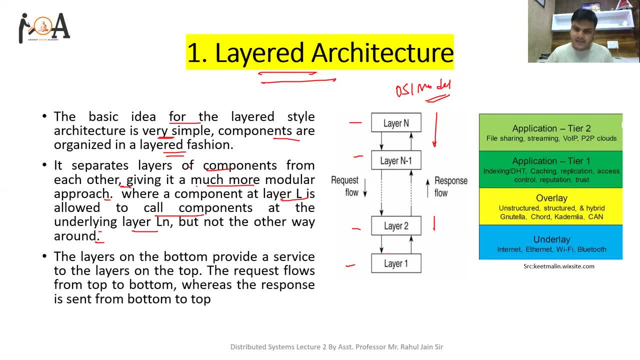 under the distributed system is mentioned, where layer one is connected to layer two, it can distribute the resources. it can share the resources with layer two, but it can't directly share the resources to layer three until and unless it is not a special case. so the layers on the bottom provide services. 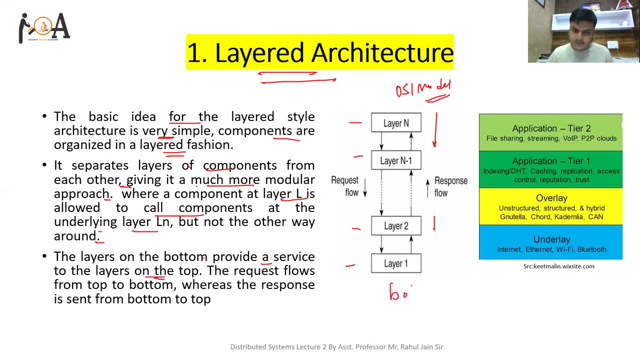 to the layers to on the top. so this bottom, bottom side layers provides provide services to the layers which are upper side. they are upper side layers, okay, and the request flow from top to bottom. so request flow would always be from top to bottom. very important point to note: from top to bottom what top to bottom request flow. 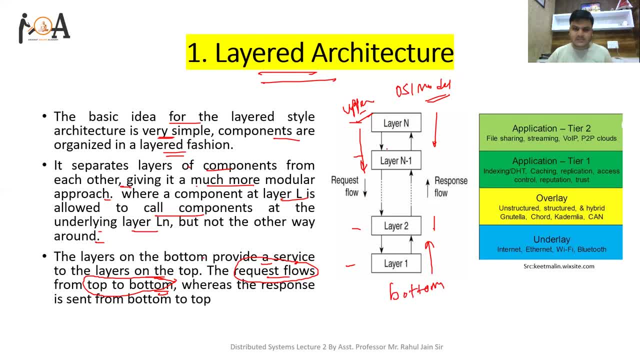 would be from top to bottom. layer n would request layer n minus one. it would request like that and response is sent from bottom to top. response flow would be from bottom to top. bottom to top would be response. layer one would provide response to layer two, layer two would provide response to layer three and till n. now you can simply see here that in 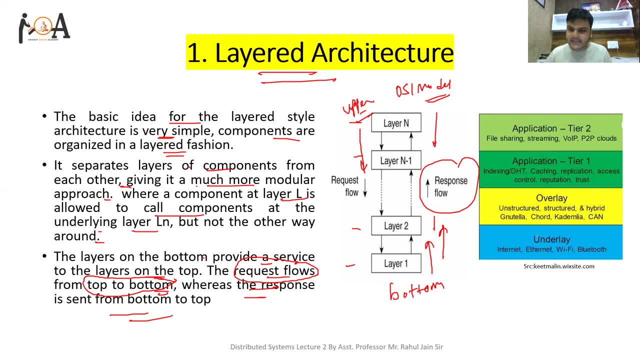 this way distributed system architecture, of layered architecture can be assumed that the bottom side layer underlay, which is generally nothing but internet, ethernet, wi-fi or bluetooth. they can provide responses like that to unstructured or structured and hybrid. Juntilla Cord Cadamelia. 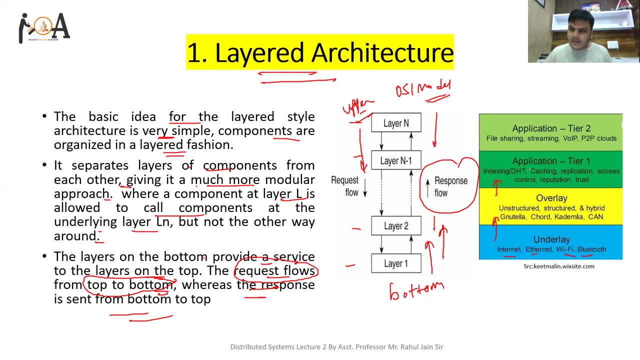 or Cairn, and further on the upper layer. it would be like: tier one: indexing, DHT, caching, replication, access control, reputation, trust and application. tier two, that is file sharing, streaming, voice over, internet protocol, p2p clouds, like that. so basically, it simply means that these services are under the layer. they are categorized like that. so request flow. 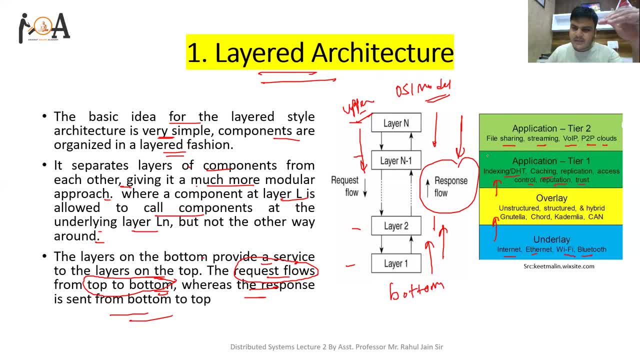 request flow would be request flow, that file sharing would be request from indexing and it would be like that. so request flow it would be from top to bottom and response flow is a response. So request flow would be from down to top, bottom to top right. so it is layer architecture. 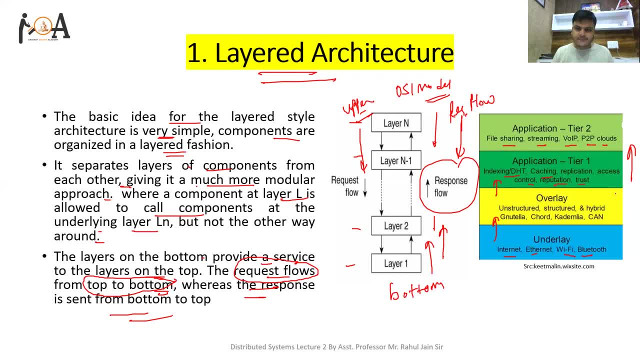 it is very modular, very simple, and if you will see here that it can, you can assume it simply like OSI model layer, right? so this is the layered architecture of distributed systems in which resources are shared layer by layer and all the request flow and response flow would be in that manner, right? the next one here is object based architecture: object. 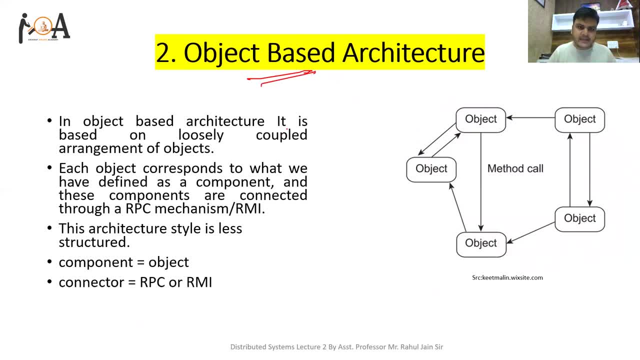 based architecture. So in object based architecture it is based on loosely coupled arrangement of objects. it is based on loosely coupled arrangement of objects and, if you will see, here each objects corresponds to what we have defined as a component and this components are connected to RPC. that 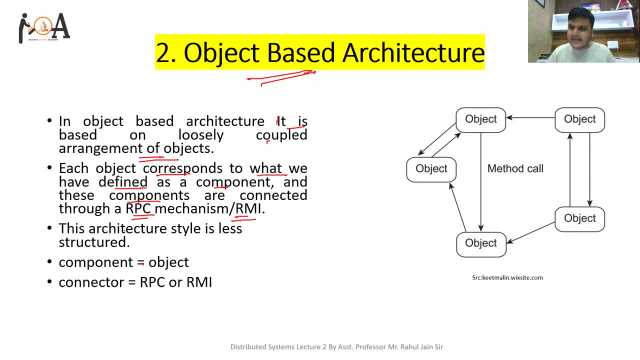 is remote procedure calls mechanism or RMI, that is remote method invocation, right and this. So, if you will see here this architecture style is less structured. the components are termed as object here and connectors are remote procedure calls or through remote method invocation. so, if you will see here these objects are there in object based architecture, the objects 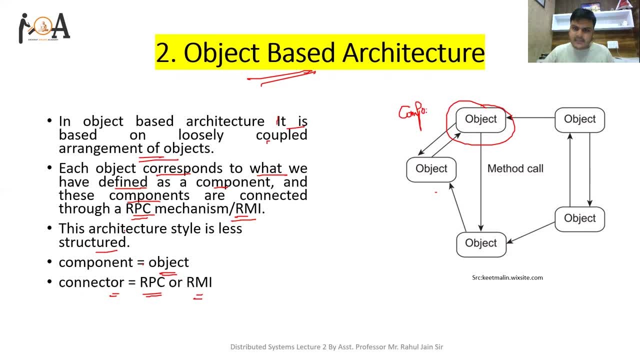 are nothing but they are components. they are nothing but they are components. or you can simply say that in easy language, that nodes, right, these nodes, these components, basically in object-based architecture are termed as objects. so these objects will communicate with each other with the help of rpc- right, with the help of rpc, that is, remote procedure calls- they can talk to. 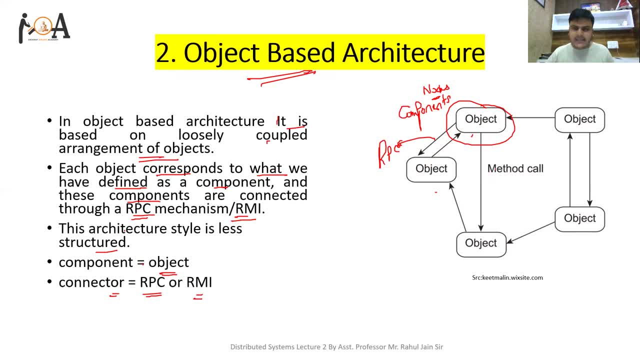 each other which is connected. but if they are not connected, they can use specialized the method which is called as rmi, that is, remote method, invocation, method call and with the help of method call they can interact with any other objects. they can share the resources in that. 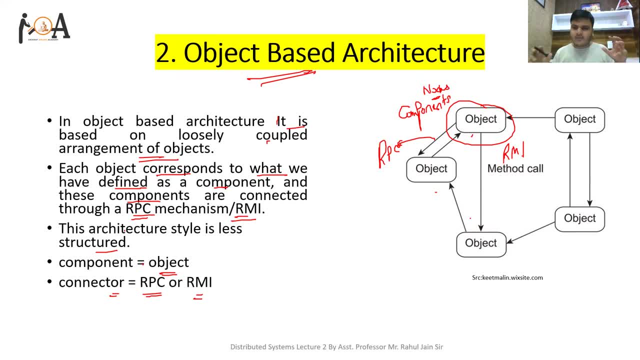 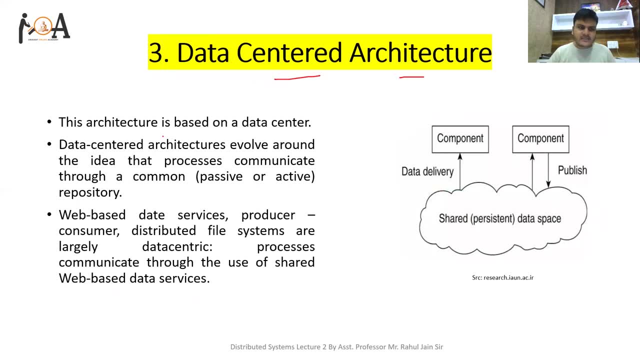 manner and such. in that manner they can work together for a common goal. okay, and if we talk about the third one, that is, data centered architecture in this, this architecture is based on a data center, a commonly shared persistent data space is there, a data repository is here. 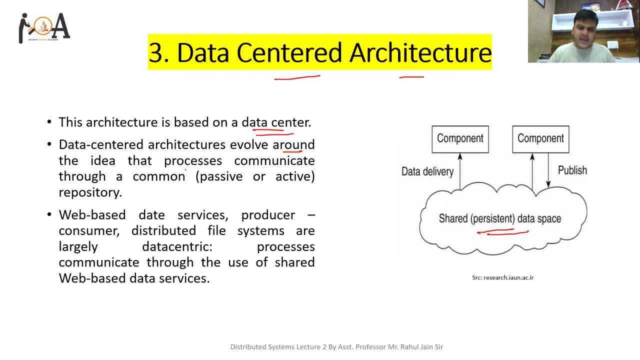 data centered architecture evolve around the idea that processes communication through common repository. this is a common repository, common repository, Munich, Munich, Munich, Munich, Munich. you can simply say that it is just simply like producer and consumer: producer and consumer problem- Okay, so producer will produce the data and it will shared in the common data space and 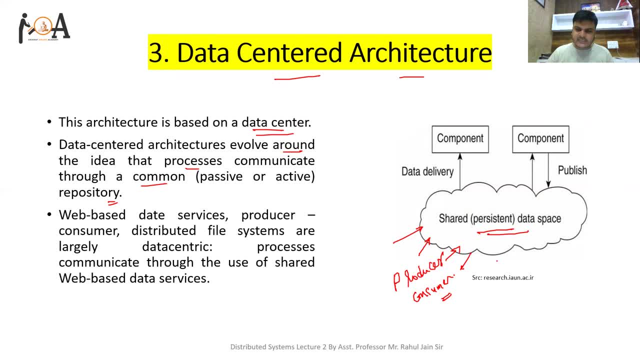 consumer will consume the data from this common data space, right? So it is just like that. and web-based data services- producer, consumer and distributed file systems- are largely data centric and the processes communicate through the use of shared web-based data services. So here you will say that we have components, digital devices, computing devices like that. 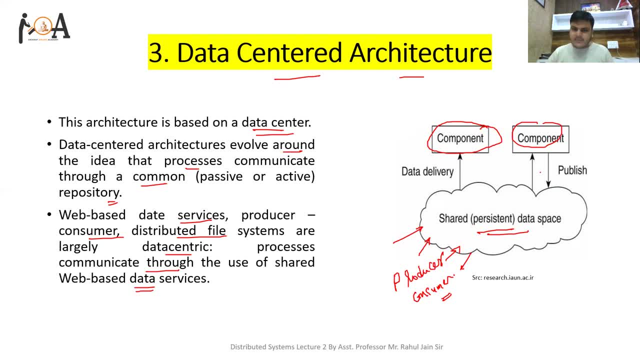 and they can publish- or they suppose they can publish- the data. They can produce the data and whatever data need to be consumed depends on the components they can consume that are throughout that. So all the resources are shared commonly here In the common repository. okay, 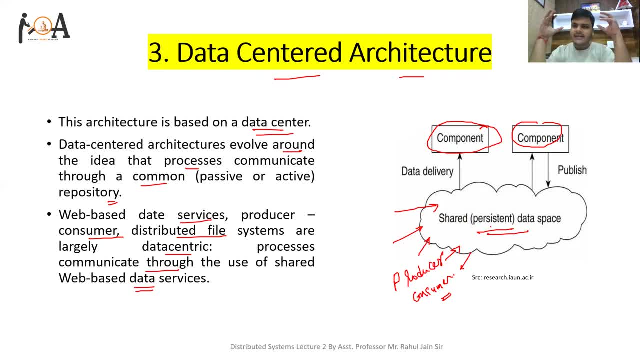 So, just like web-based data services in which all the data storage is common, whatever query would be there, it would be provided by searching from that common data storage and that will be provided to the. that would be provided to the whoever have requested that right. 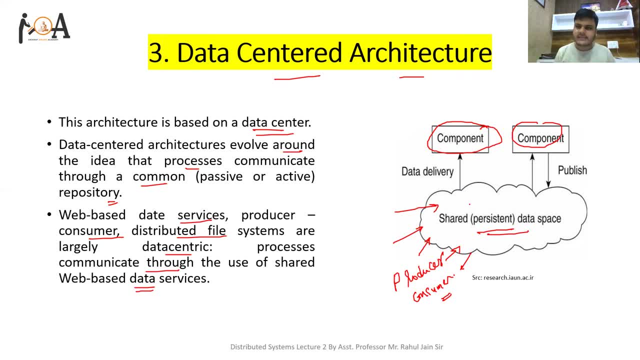 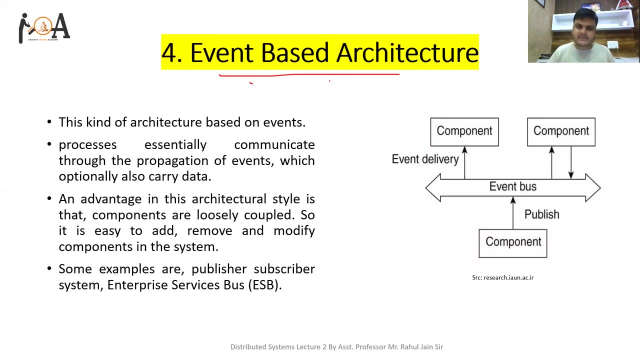 So it is the data centric architecture. The main crux of this architecture is common repository, from where each and every resources is provided And each and every resources is shared in that common data space. The next one here is event-based architecture. event-based architecture. 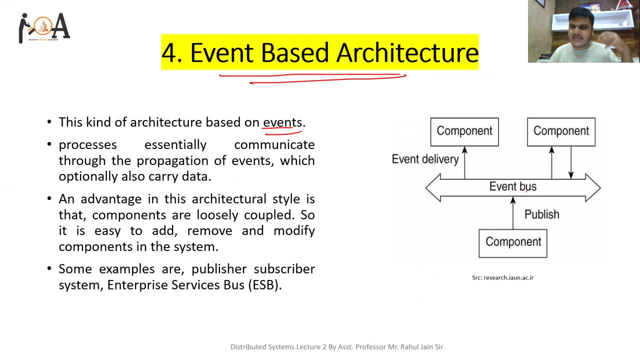 So the kind of architecture based on events in this, events are occurred, events are occurred and that events will be shared to the bus. that events would be shared to the bus, So each and every component, each and every component which is attached to this bus will. 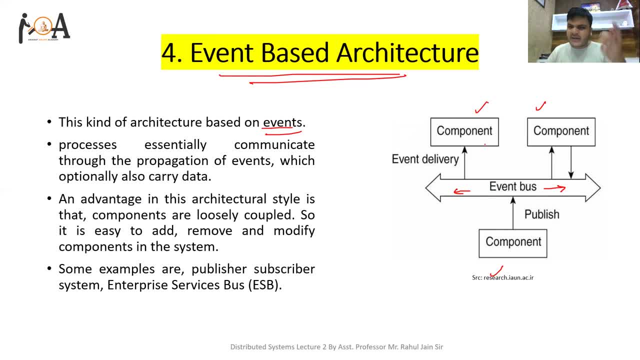 get to know that event is occurred. Now, whichever component want to attract, whichever component want to get that event, would get that event throughout that bus right. So each and every component here would know that event is occurred via this bus system. A bus system is there in which the propagation of event would be occurred, and many components. 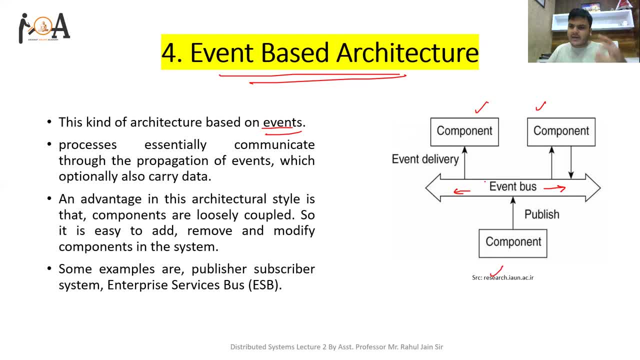 are attached to it. So whichever component required that event will get that event directly from that bus. Okay Processes essentially communicate throughout the propagation of events, which also optionally carried data. It can in many cases, sometimes it can also carry the data. 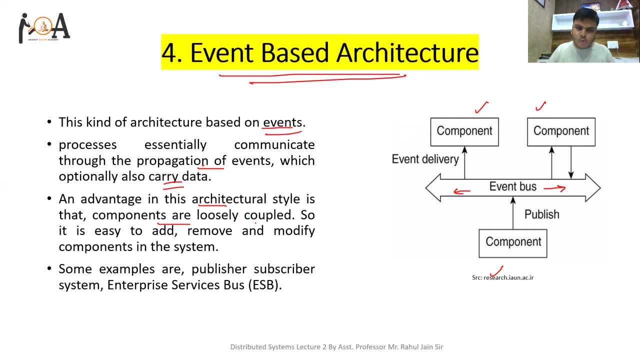 An advantage in this architecture style is that components are loosely coupled So it is easy to add, remove and modify components or systems. So in in this system, in event based architecture, the components are very easy, very loosely coupled, So whenever you want to add or whenever you want to delete, or whenever you want to modify, 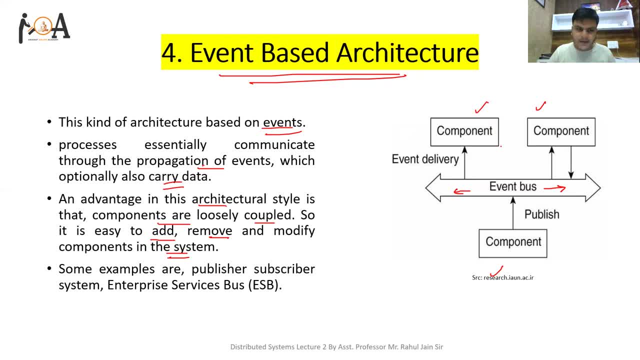 the component. we can do it easily as they are loosely coupled And if you'll see the components here, basically these components can't interact with other component here. If they want to interact with the other component, they need to go with the, they need to subscribe. 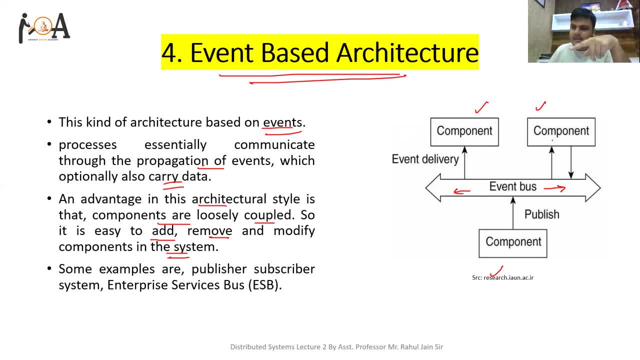 this event and, with the help of that event, they can interact or share the resources with the other component, like that. Okay, And some examples of this event based architecture are publisher subscriber system and enterprise services bus system, ESB. So the crux of event based architecture is propagation of a common event throughout. 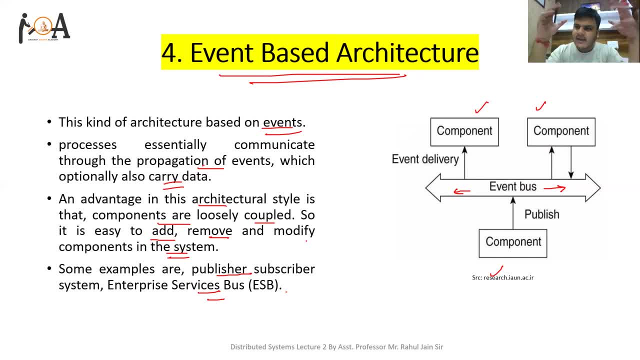 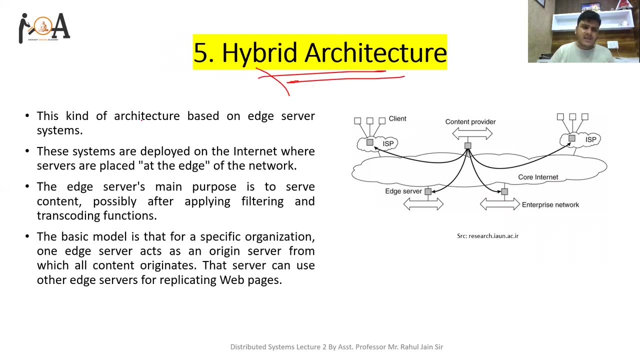 that event. Other components will observe that it event is occurred and if they require that event, they will attract that event. They will capture that event throughout that common bus system. Okay, And the next one here is hybrid architecture. Hybrid architecture, This kind of architecture based on edge server system. edge server system. edge server system. 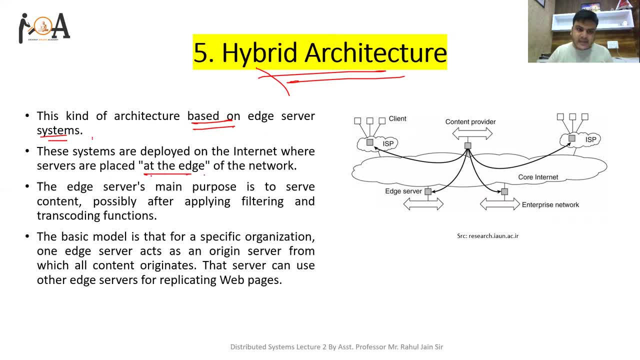 This system are deployed on the network where servers are placed at the edge of the network. Servers are placed at the edge of the network, right, You can see like that, And the edge server's main purpose is to serve content, possibly after applying filtering. 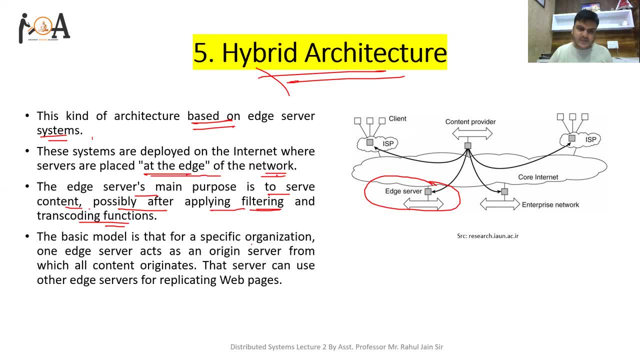 and transcoding functions. The basic model is that for a specific organization, one edge server acts as an origin server from which all contents originates. That server can use other edge servers for replicating web pages as well. So in hybrid architecture it is using client based server as well as it is using peer to 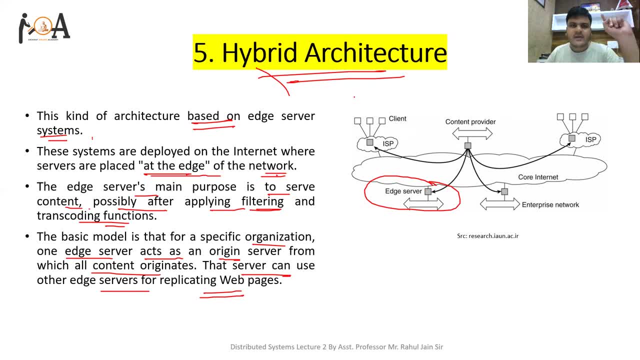 peer system. So in our first lecture, in our first lecture we have discussed there are two types of mainly architectures. One is client server architecture, in which client will request the server and server will respond to the client right. And second is peer to peer system in which the task, the resources would be equally divided. 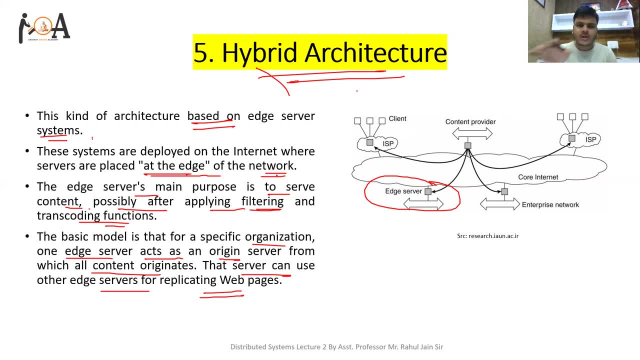 between the peer systems and they will collaborate for a common goal. So the combination of both is under hybrid architecture- You can see here- in which edge servers are placed at the edge of the network- and main purposes. It can filter, It can transport the functions and resources which is required to any client or to any